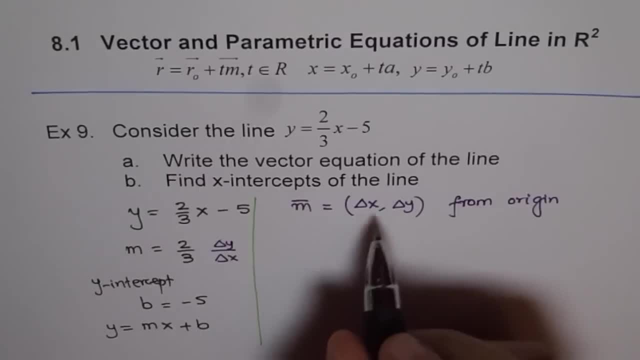 Origin. Okay, so for this equation, M is equal to 3 over 2, right? so that is how you know. if you have equation in slope intercept form, You can straight away write the direction vector correct: 3 over 2. To give you a good idea of all this, let me say this: so we are saying that 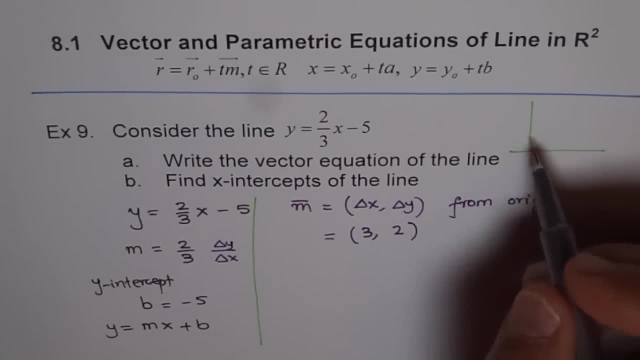 Our line Direction vector from the origin is 3 over 2, so this is like 1, 2, 3 and then this is 1, 2, Then that's the point: 3 over 2 and from here to here that denotes the direction vector M. 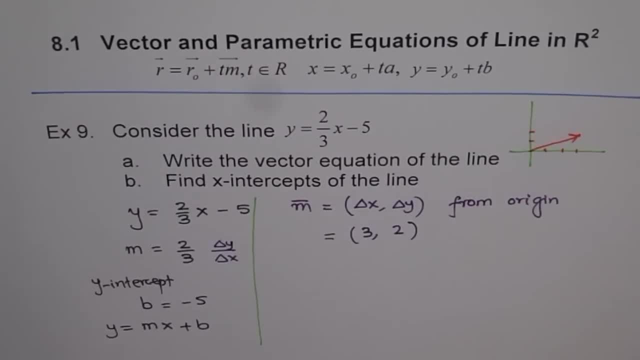 in vector equation of the line. okay, Now for writing equation of a line in vector Form, we need direction vector and a point. so the point which we are going to use here is the y-intercept, correct. so the point which we will call as r0 is equal to. 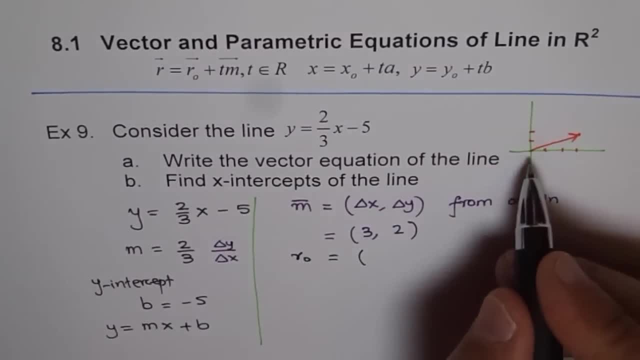 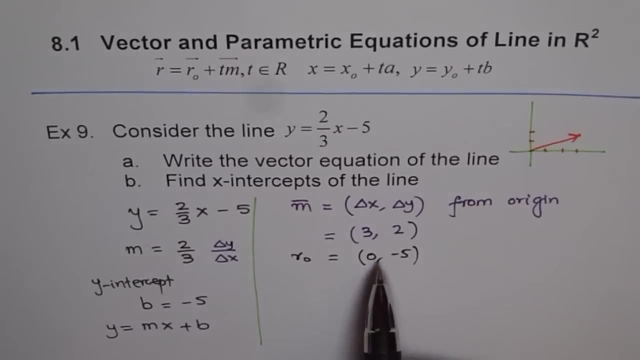 the value at y-intercept, which is At 0 minus 5. so we say 0 minus 5. the y-intercept given in this equation will be used as our point on the line, correct, and Then we can write r0. so r, r. the vector equation say r is equal to r0, which is the point: 0 minus 5. 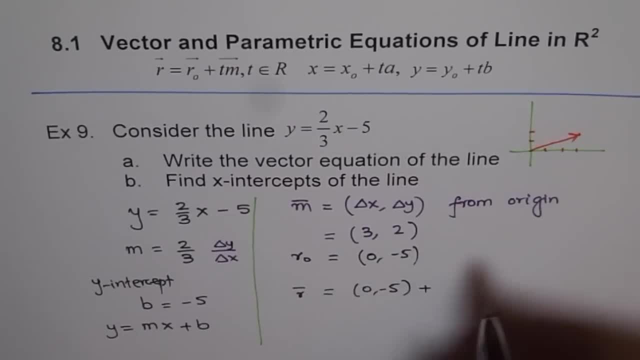 plus any scalar multiple in this direction, correct? so that is, We can use any symbol here, right? normally we are using T, So I'll use T for the time being, but it could be any symbol, right as UV, whatever you feel like. Well, so it is T here for the moment. 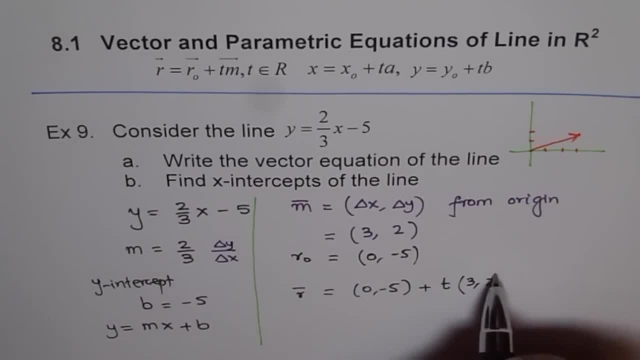 and then the direction vector, Which is 3 comma 2, now T, here belongs to set of real numbers, correct, so that it shows all The points in this direction, right in this direction. but our points and the line which we are talking about has a y-intercept of minus 5. so 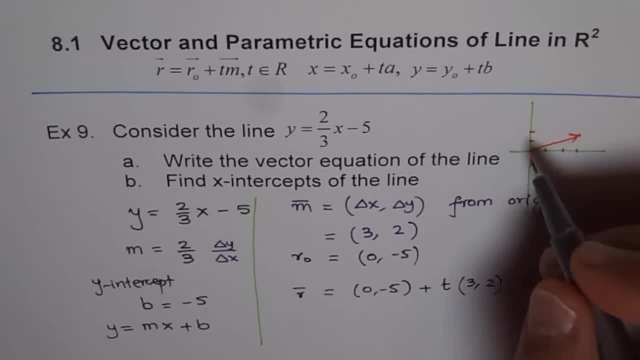 Let me just extend it and try to give you the point here. so this is like plus 2 here and now we say this is 1, 2, 3, 4, 5. so that is the point Which we are looking for. so that is the y-intercept and 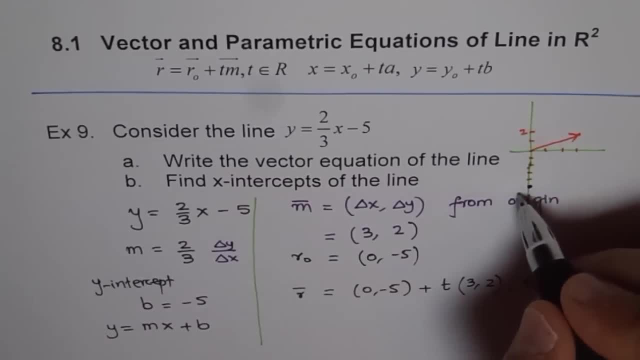 You know. so, basically, we are going to draw a line Which is parallel to this. from here, You see that you understand the concept. so here We have to go, three units to the right and two up right. so we get a point like that, And let me do it in a different color. so this line, 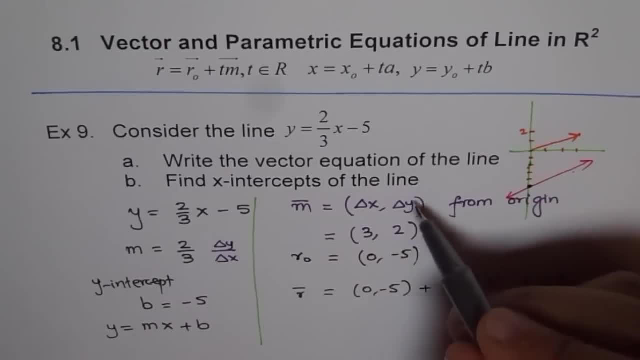 is the line which we could draw Using our vector equation, right? so that's the point: 0 minus 5, Correct. so this point is 0 minus 5, correct. and then from here we go: 3, 2, so that means see 1, 2, 3 and 1, 2, and we reach a point here and then 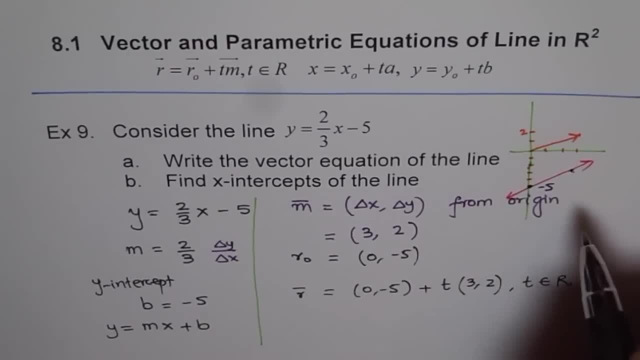 Connected like that. now this T could be any multiple, right. if it is 1, then we go 3, 2. if it is minus 1, We could have gone this side also, right. if it is like 2, then 6, 2, so we can go 6, and next point will be here. like that, there were so many points on the line. 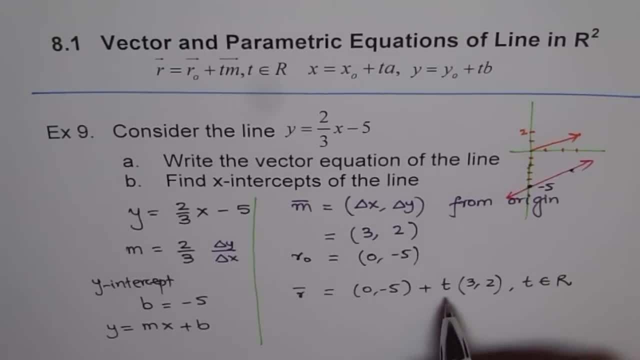 so this factor T belongs to real number, ensures that line is a set of. Let me write that in a different ink: Line is a set of infinite points. right line is a set of Infinite points In the same direction, right, and That value of T and shows that same direction, do you see? you just change the value of T. 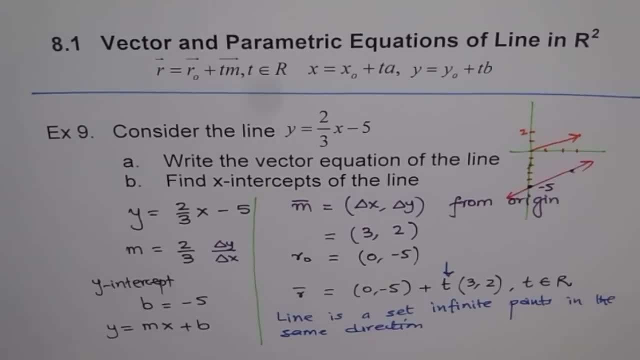 It could be 1, 1 point 1, 1 point 2, 1 point 3, 10, 111, whatever right, But gives you all the points in the line. It could be negative, positive, all real numbers, correct. so that is what it is. 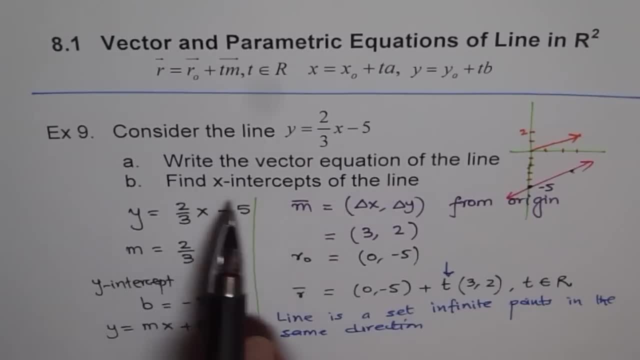 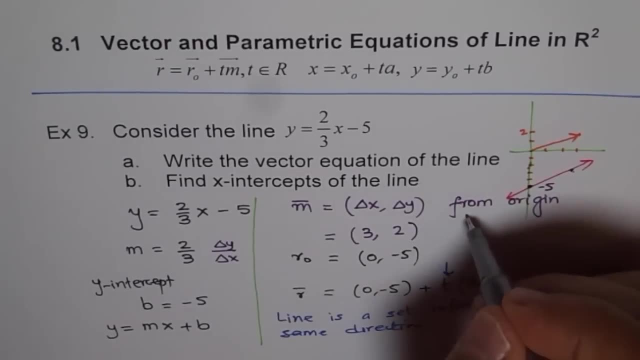 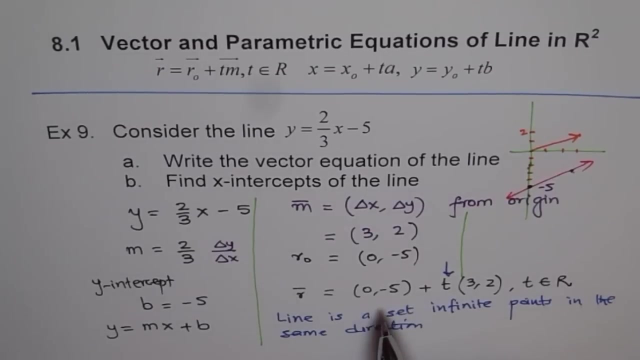 So I hope you understand that part. and now let's look into the X intercept of the line. so to find the x intercept. so I'm running out of space here, so I'll just make a room here. so x intercept means that y equals to 0, right? so we are looking for a point where y is equal to 0. 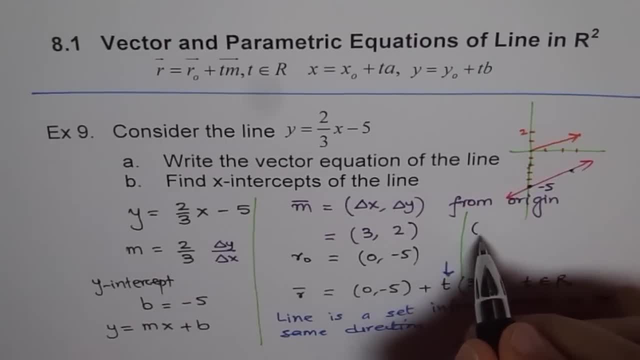 and we'll find some x intercept. so let's say the x intercept happens to be at x comma 0, right, because that's the y value and it has to go through this point, right, 0. that's the equation. so we get 0 minus 5 plus t, 3 comma 2, right? so the idea is to find what value of t will give us. 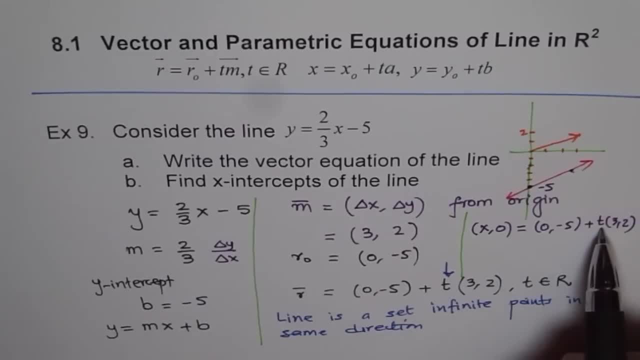 the 0 y value. the same value of t will give us the x value, do you understand? so? so the y value 0 can be equated as 0, equals to minus 5. see, we are splitting the equation into its variable x and y. okay, so in a way, we are writing the 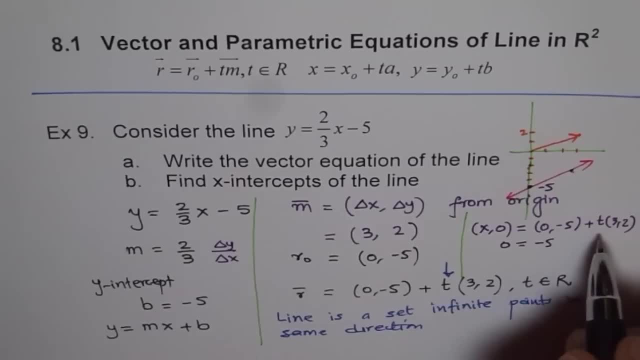 parall해설- parametric form. now, okay, or we can just expand and write and then see: okay, so we could. yeah, okay, so well, let. because i started like this, let me do it like this: now: zero equals to minus five plus two t right plus two t right from here. we know t is equals to: 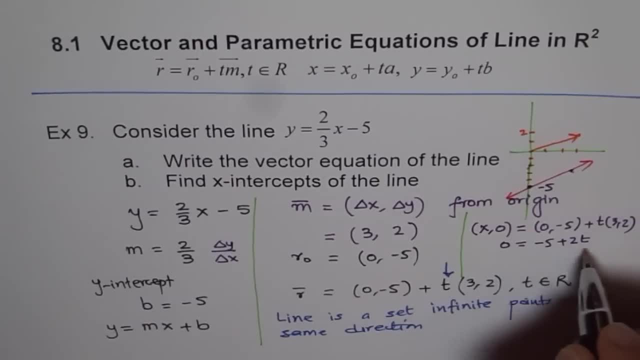 five over two. correct t is five over two. so this gives us t equals to five over two. so the x value will be: so x will be equals to zero plus five over two times three. zero plus five over two, t is five over two times three. so 15 over two is our x intercept point. do you see that? so wherever it, 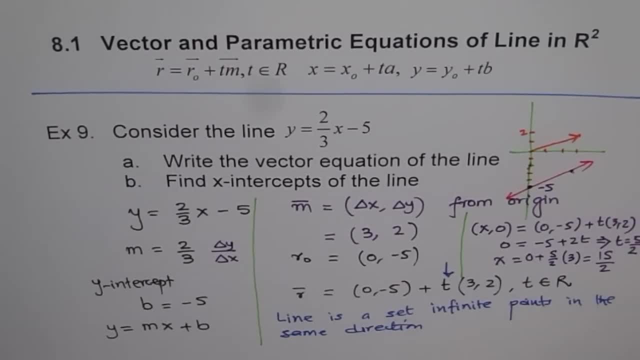 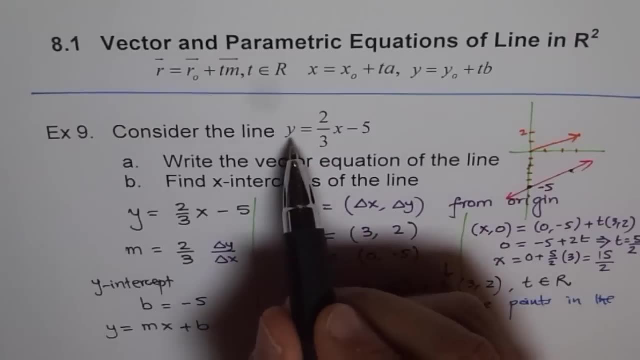 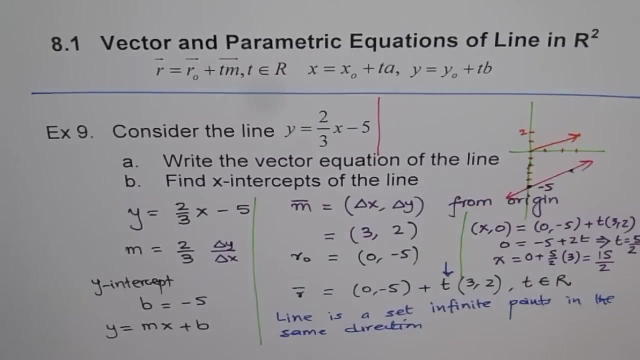 crosses, it'll be 7.5 the value of x intercept. okay, now that's how it is going to be. even if you calculate from here x intercept, if you place y equals to zero. let's do it here also, okay, so i'm just giving you different. 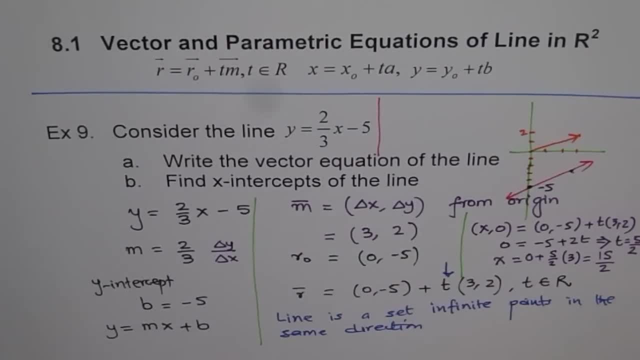 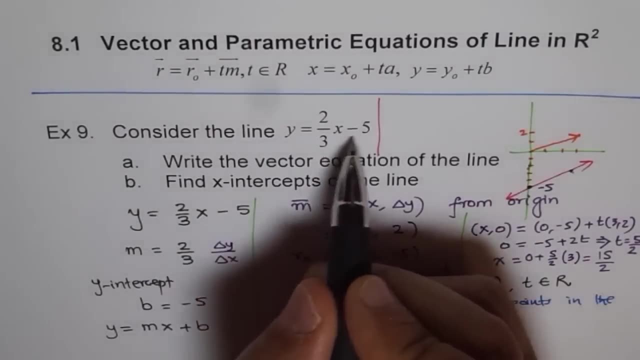 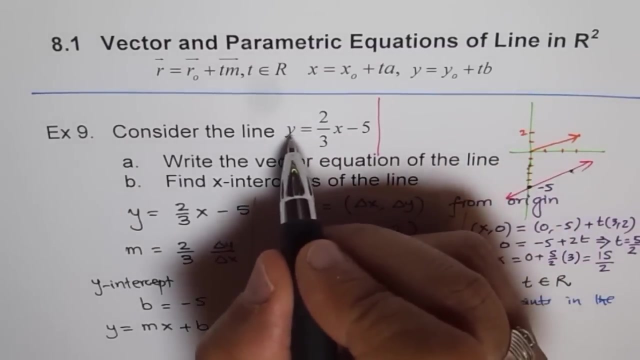 scenarios, trying to make you understand and link the y equals to mx plus b with the, the vector equation. right now here: if i put y equals to zero and solve for x, let's say then: and i multiply by three. so okay, let's do that. let's equate: y equals to zero and then becomes: